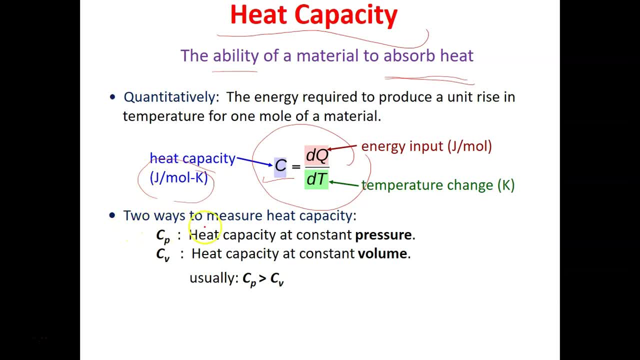 work out your heat capacity. So there are two ways to measure the heat capacity. The first one is the heat capacity, constant pressure. This is measured at constant pressure, And the second one is cv, in which the heat capacity is measured at constant volume. So most of the time, 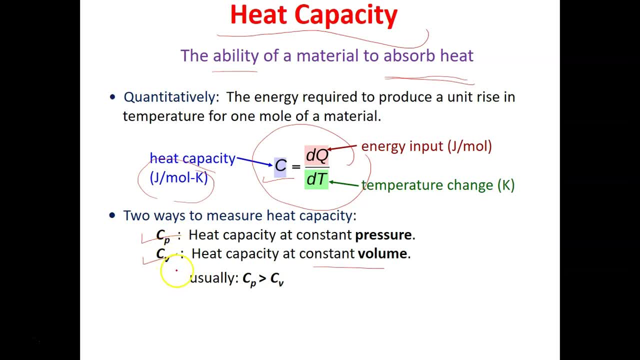 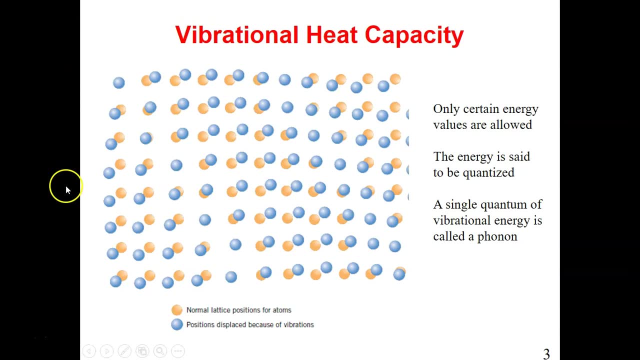 cp is always larger than cv, All right. next, we have vibrational heat capacity. This is new to you. So what is it actually? So you all know that atoms in solid materials, they are constantly vibrating. They are constantly vibrating at very high frequencies. 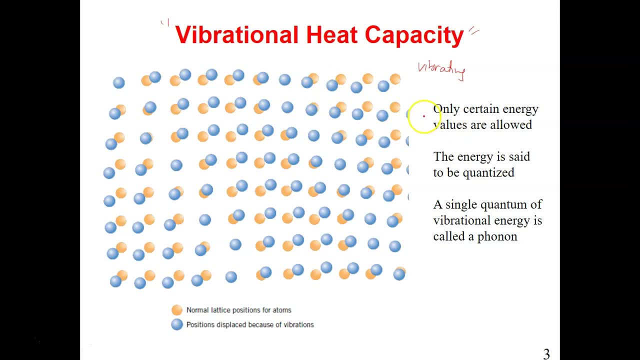 Vibrations of the adjacent atoms. they are actually coupled by the virtue of the atomic bonding. So, as you can see from this figure here, it shows many, many small balls. So what does it represent? So the blue color, all of these, they represent atoms And the blue color actually represents 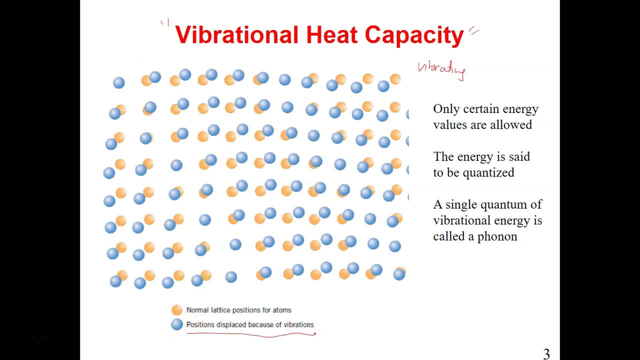 the position of the atom displaced due to vibration, And the orange color. this is the position, or the normal lattice positions for atoms. Okay, so due to this vibration, the atom is displaced or delocalized into a new location. So the vibration, they happen in a way that traveling lattice waves are produced. Now, this whole thing it shows. 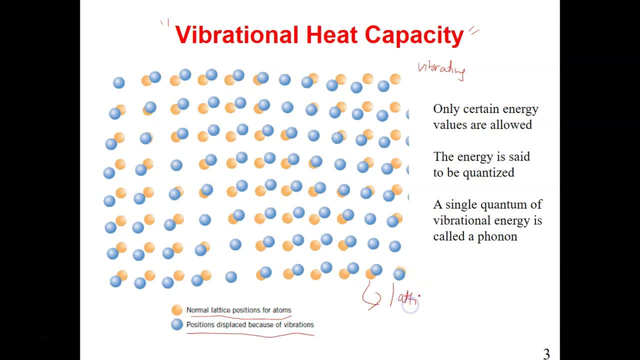 traveling lattice waves, This whole thing, the dislocation, we call it lattice waves, So this also can be thought of as elastic waves, Or we can also call it as sound waves. So these waves, they have short wavelengths and very high frequencies. 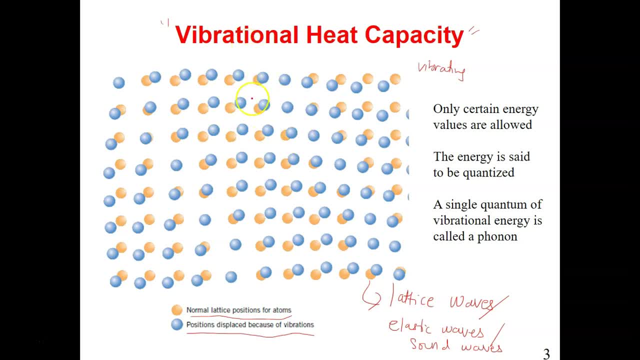 So the vibrational thermal energy for any material actually consists of a series of these elastic waves, or lattice waves, that have a range of distributions and frequencies And that only certain energies are present. They are also known as quantum waves because the quantum energy values are allowed. 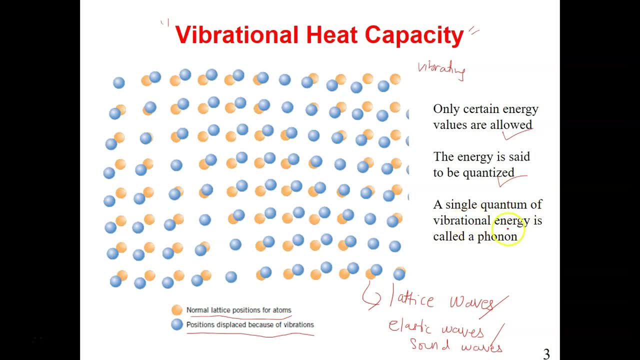 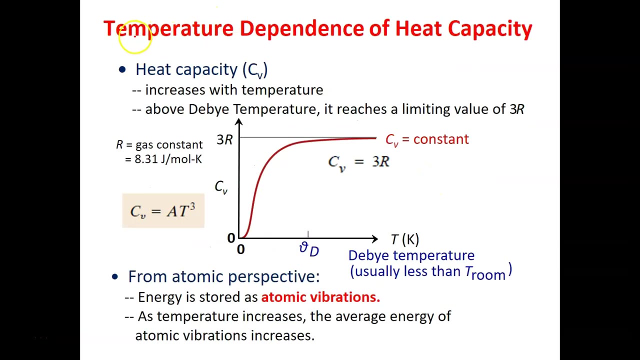 And the energy is to be quantized, And a single quantum of vibrational energy is called a phonon. So these elastic waves, they actually participate in the transport of energy during thermal conduction. Let's look at the next topic, what we call as temperature dependence of heat capacity. 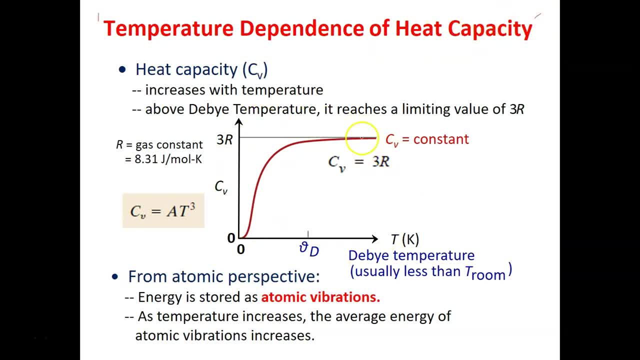 All right, Alright. so if you look at this graph here, so this figure actually shows the variation of temperature, of vibrational contribution to the heat capacity at constant volume, which is Cv. Okay, so you can see that the Cv is zero when at zero Kelvin and it rises rapidly, rises very rapidly with temperature and this actually corresponds to the increased ability. 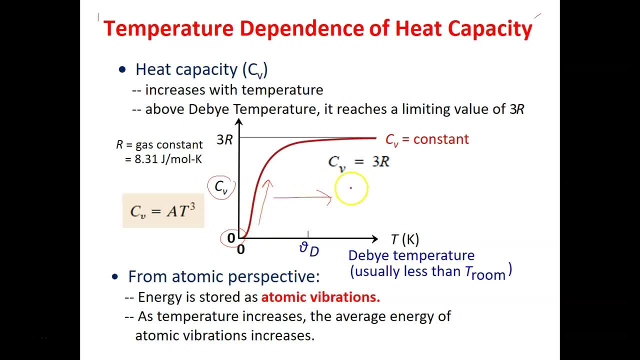 So this actually corresponds To the increase of the ability of the lattice waves. Okay, with increasing temperature and at low temperature. so we consider this as low temperature, At low temperature, At low temperature. the relationship between Cv and T and E is given as this: 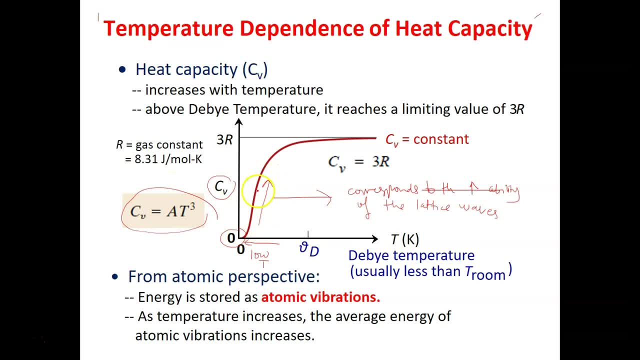 This is the relationship at this rapid increase or lower temperature, Where A here what is A? A is temperature independent constant. So this is a constant, All right. And this one, This one is what we call as Debye temperature, So this usually less than the room temperature.